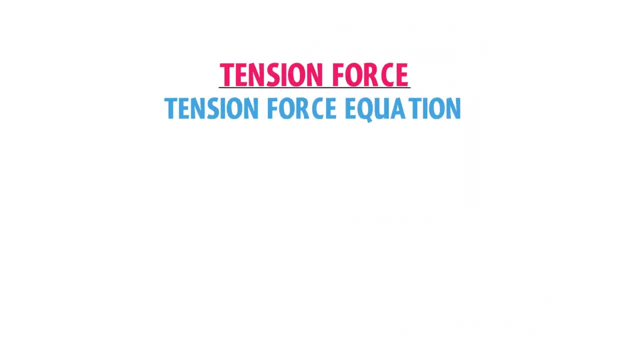 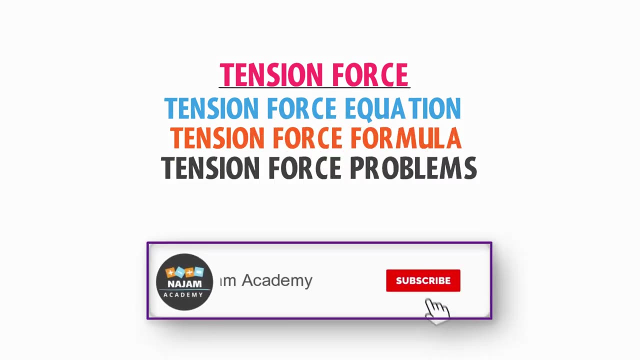 Tension Force, Tension Force Equation, Tension Force Formula and Tension Force Problems. Before starting the lecture, click on the subscribe button and get access to our 100 tough conceptual lectures for free. Firstly, you should understand the easy concept of tension. 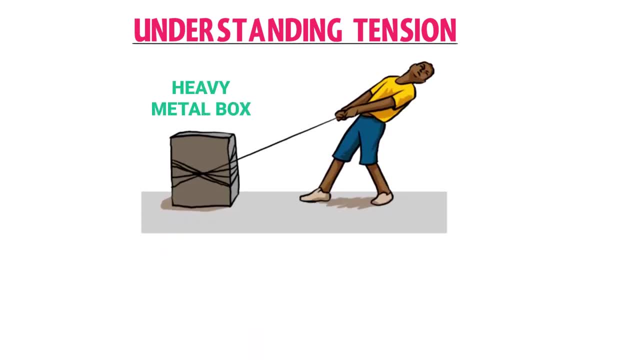 Let's consider a heavy metal box and a string or cable is wrapped around this object. You are trying to pull this heavy object in this direction by the help of this rope or cable. Now, here are some interesting points which you must learn. You are standing here while this heavy box is there. 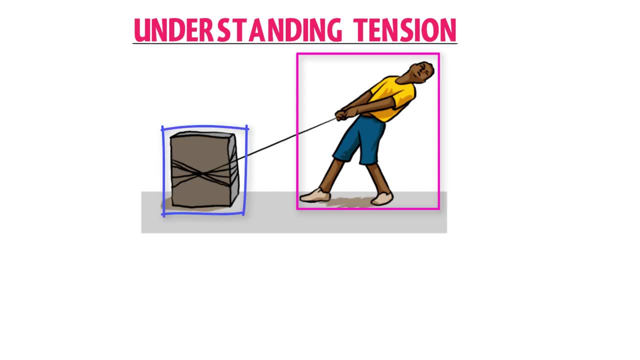 It means there is enough distance between this heavy object and you To ask you: how can you push this heavy box from a long distance, and are you a magnet to attract this heavy metal box? Well, your answer would be no, I am not a magnet, but I am pulling this. 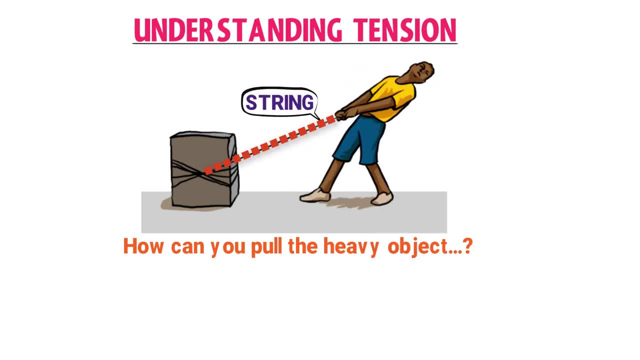 heavy object by the help of this string or cable. Thus here we learn that you can pull this heavy object at a short distance and reach the object from a long distance, or reach the tauила. Thus here we learn that you can pull this heavy object at a short distance and reach the tauila. 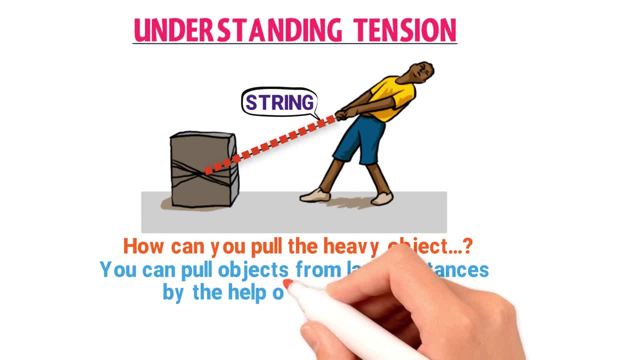 objects from long distance by the help of string or rope, without touching them. Now, what magic is lightning and this rope? Well, you are pulling the string in this direction. You are not pulling the object. When you pull the string, you exert force on it in this direction. The string translate or transmit your force. 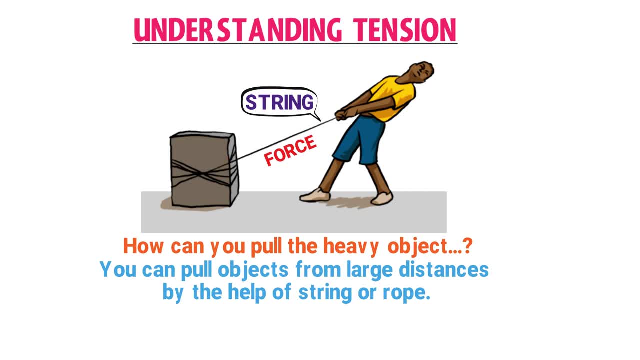 to this heavy object. As a result, this heavy object is pulled and this direction. To simplify it further, let me teach you Here. we assume that the string is massless means the mass of the string is zero, which is not true in real life. 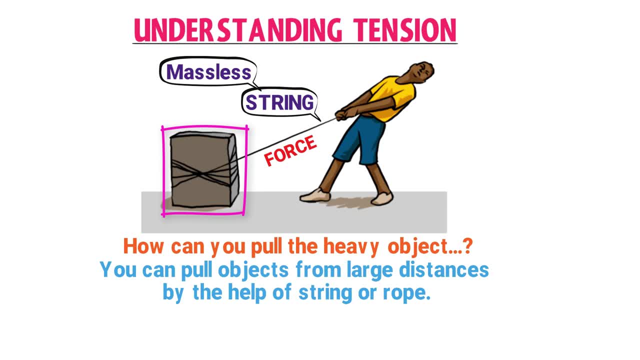 But in front of this heavy metal box, the mass of this string or cable is very small, So we neglect it. Now, for example, you exert a hundred Newton force on this string in this direction. String will translate this hundred Newton force to this heavy 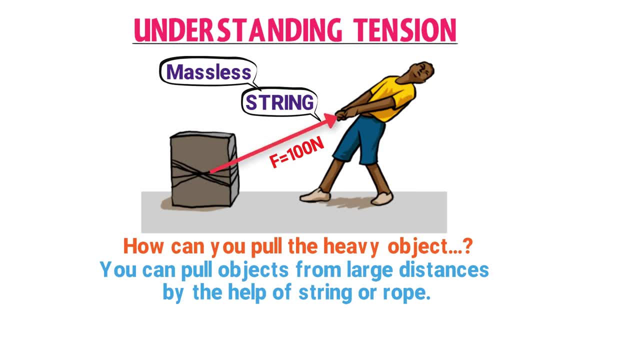 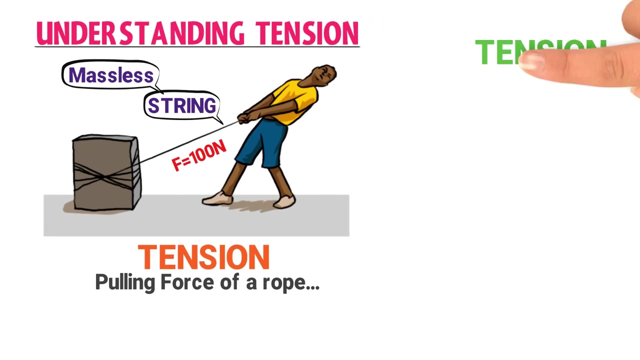 object and it is pulled away. Now, this hundred Newton force and the string or rope that is translating, is given a special name in physics, known as a tension. Therefore, whenever you read or listen tension, always say that tension is the pulling force of a string or a cable. Remember that. 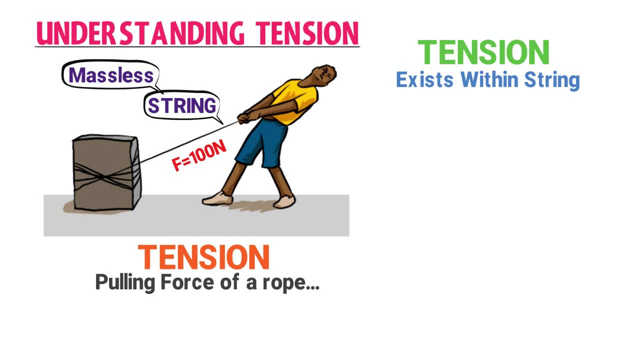 tension exists within a string or cable and it is applied by the string. For example, in this case, tension exists within this rope and it is applied by this string on the heavy metal box. Also, remember these two bonus points about tension. Firstly, tension is a lifting force. For example, consider a mass M suspended by a string. 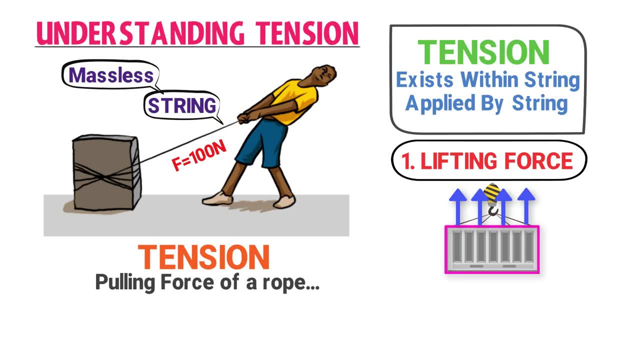 Here, the tension within the string is lifting this heavy object in an upward direction. Secondly, tension is a pulling force. For example, you pull this heavy metal box in this direction By the help of the rope. our tension exists within the string. Remember that tension cannot push objects. Or you can say that: 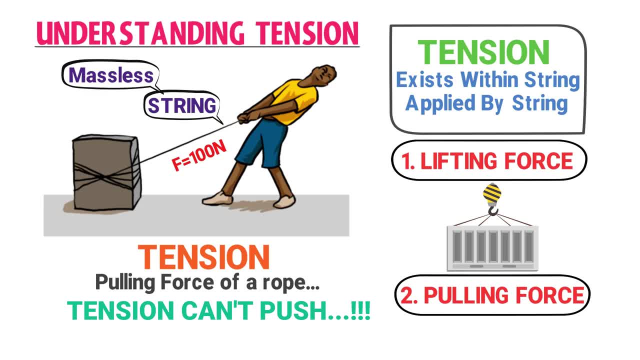 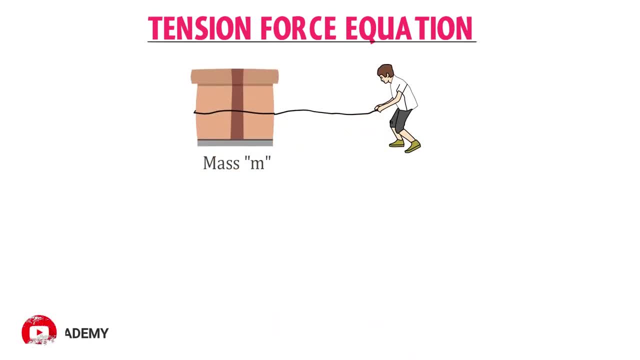 tension cannot act as a pushing force. Let me also derive the tension force equation. Let consider a mass M and you pull this mass in this direction by the help of a string. The net force on this mass would no longer be zero and acceleration every second is equal to zero. 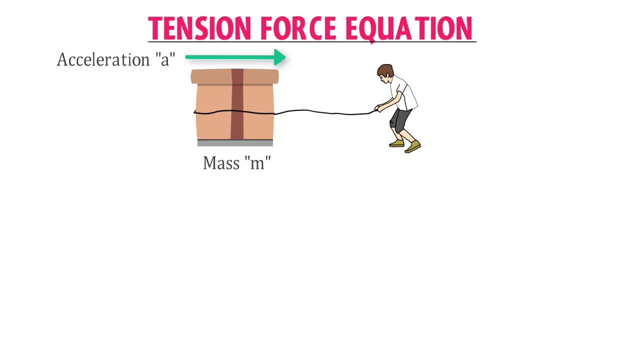 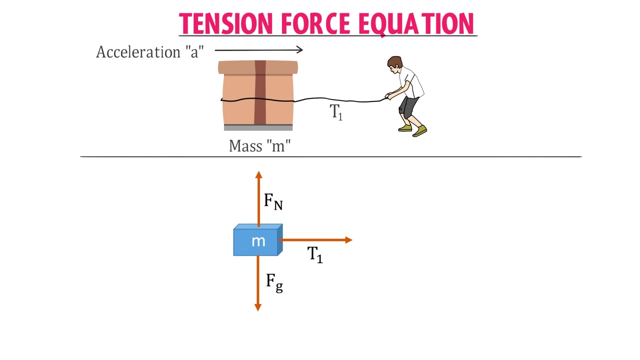 Therefore, the mass M will be produced in this direction. Note it down that acceleration A is produced in this mass M due to tension T1 in this string. Now let me draw a freehand diagram for it. In this freehand diagram we can see that 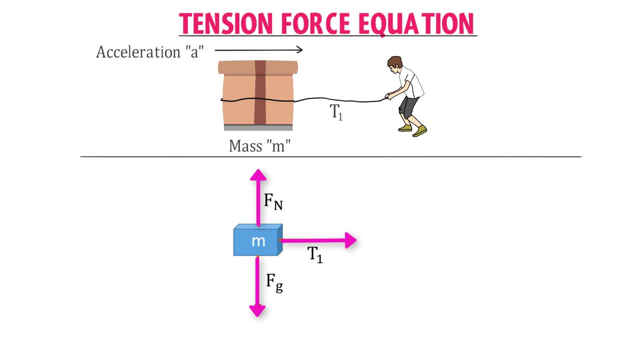 there are three forces acting on this mass. The downward force is the gravity force, RFG. Here you look at the numbers again. Hence, in general, there are three forces, as shown in the diagram. Firstly, gee gear is the force that accelerates this mass up. 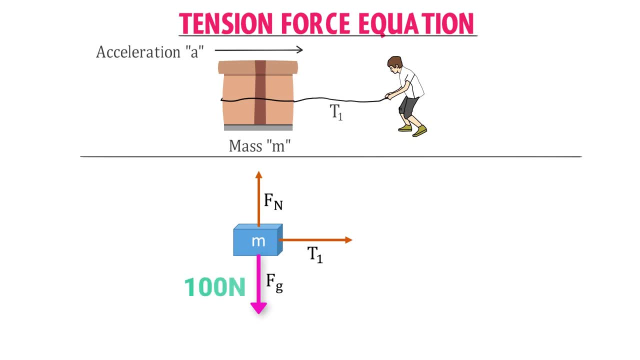 Secondly, gear is a vertical force. R is a potential force which uses this force to pull an upward or negative force in this direction. And thirdly, here you can see that gear is a negative force which uses this force to force, and upward are in opposite direction. Hence the net vertical force. 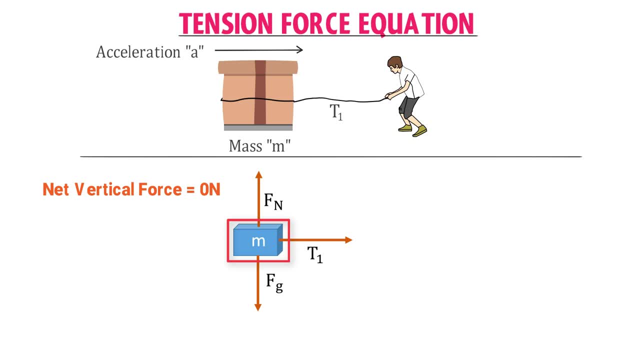 on this mass M is zero. Thus there is only one force, our tension T1, acting on this mass M in this direction. Remember that we neglect the fraction force of ground. Tension has no formula. We can derive the formula of tension from Newton's second law of motion, which is: f is equal to m into air. It means if: 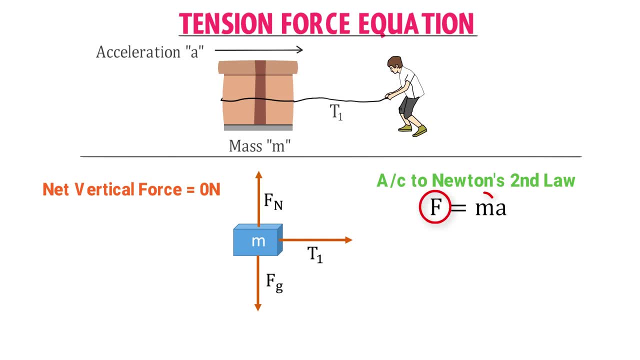 force f is not zero on mass m, acceleration air will be produced, and an object Here, tension T, is a pulling force. it produces acceleration air in this mass M. Thus we can write Newton's second law of motion n infectionsouter subscribed terms of tension, as t1 is equal to m into air. This law means that if the net tension t1 is not 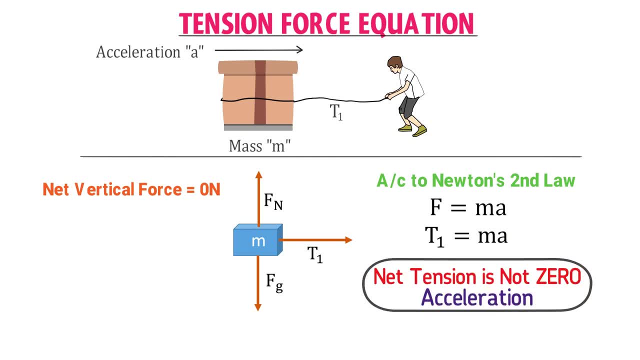 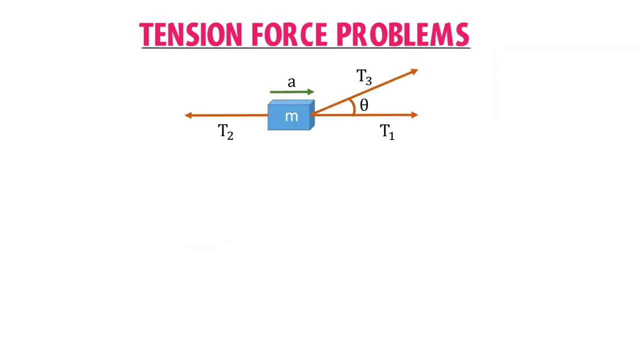 zero acceleration air will produce a mass m. You can say that net tension t of the string or loop always produces acceleration air and mass m attached to the string or cable. Now let me teach you tension force problems. For example, consider that you are pulling. 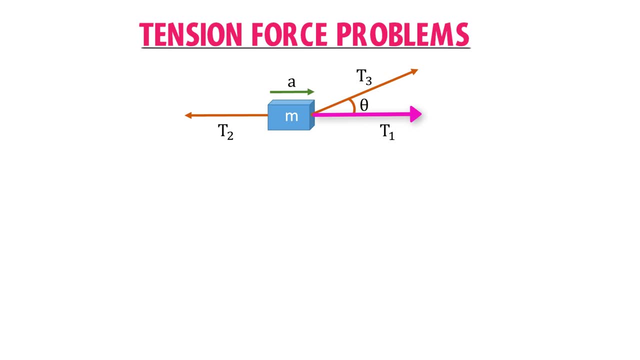 this mass m by the help of string. in this direction. Your cousin is pulling the same mass m in opposite direction. Suddenly your brother comes and he starts pulling in this direction. As a result, acceleration air is produced in the mass m and in this direction. Let the tension in your string is t1, the tension in your cousin string. 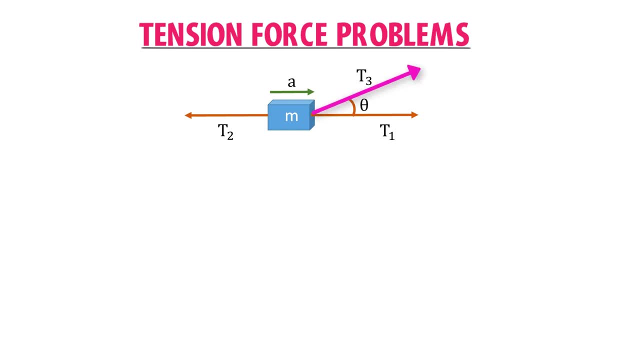 is t2, and the tension in your brother's string is t3. The tension t3 makes angle theta with the horizontal tension t1.. Now let me resolve tension t3 into its components. The y component is t2, and it doesn't produce any vertical motion or any vertical effect and mass m. But 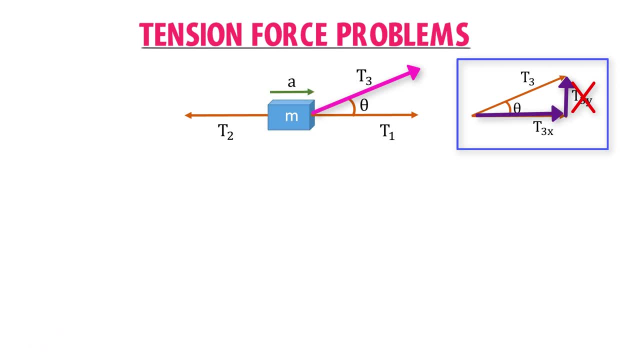 the horizontal component t3 sub x is acting on the mass and it produces acceleration air and this mass m. Using trigonometric ratios we get: t3 sub x is equal to t3 cos. theta Tension t3 is acting on this mass m in this direction. The horizontal component of tension, t3 sub. 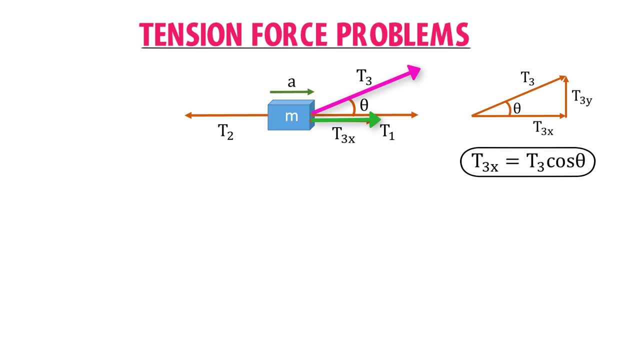 x is also acting on this mass m in this direction, While tension t2, is acting in opposite direction. Thus net force on this mass m is equal to plus t1, plus t3 sub x minus t2.. t1 and t2, 3 sub X are in same direction, so I put plus sign with them. t2 is an opposite. 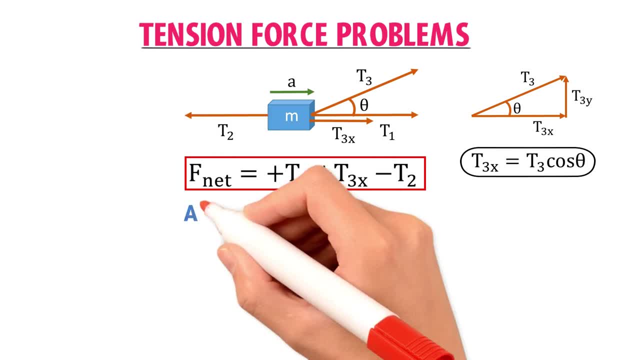 direction. so I put negative sign with it. now, according to Newton's second law of motion, F is equal to ma. put this net force and this equation- I get t 1 plus t3 sub X minus t2 is equal to M- into a. no rearranging this equation, you can.